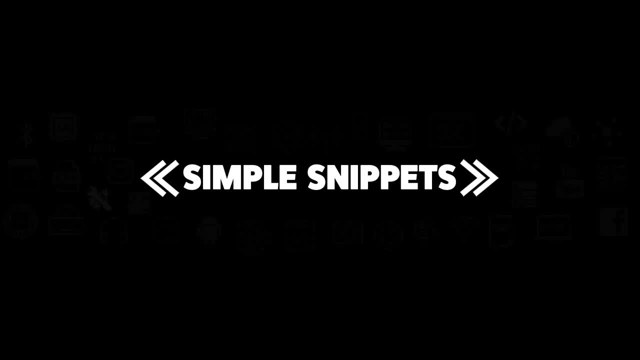 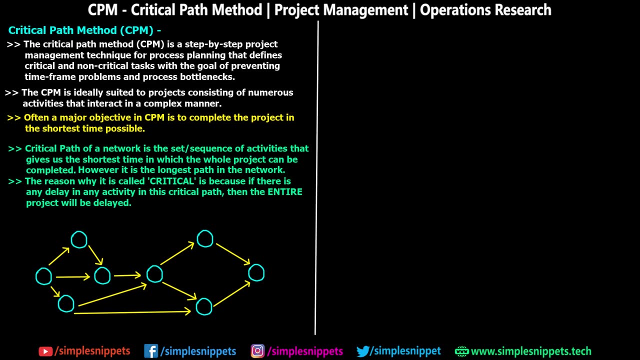 Yo, what's going on guys? Tanmay, here for Simple Snippets and welcome back to another video tutorial under Operations Research, especially the Network Analysis, Network Diagram, CPM and PERT subtopic. So in this video tutorial we are going to be taking a look at the critical. 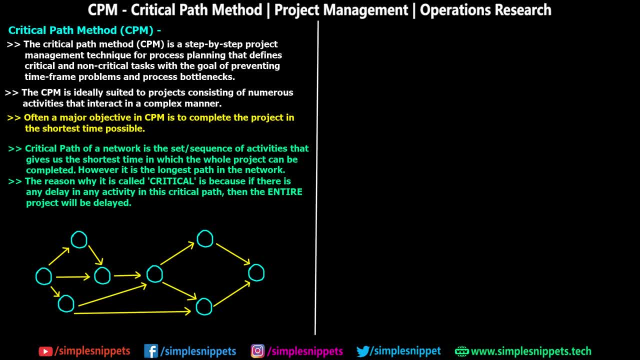 path method, that is known as CPM method, And we'll also be solving a numerical based on this technique. So in the previous couple of videos we've known what is a network diagram, what is network analysis. we saw different numerical examples on network diagram. So 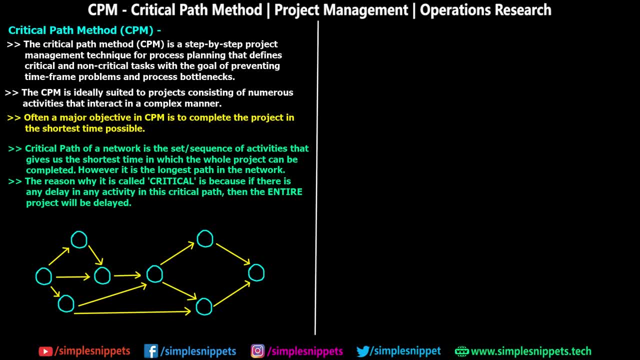 if you don't know what they are, you should definitely check them out first, And then CPM will be very easy to understand. But now let's take a little bit of theory on critical path method, And if you want to skip this theory part and directly jump to the numerical 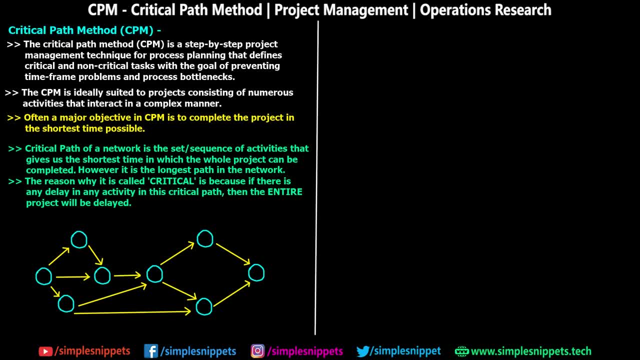 you can see a timecode where you can directly skip to the problem which we have solved. But if you don't know what is critical path method- that is why exactly it is used- just give two minutes and you'll understand it. So let's take a theory view. So the critical. 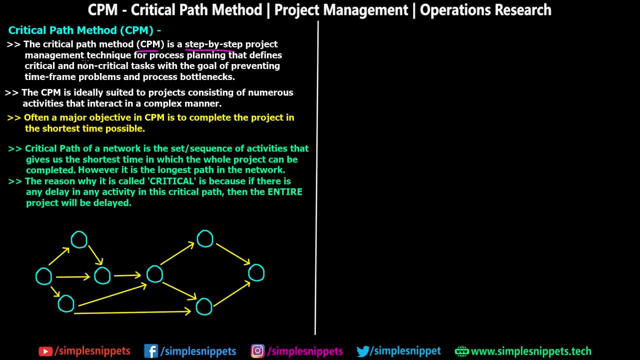 path method, known as CPM, is a step by step project management technique for process planning that defines critical and non critical tasks with the goal of preventing timeframe problems and process bottlenecks. So this is sort of like a very theoretical, very formal definition of critical path method. But to put them in simple words, what happens is: 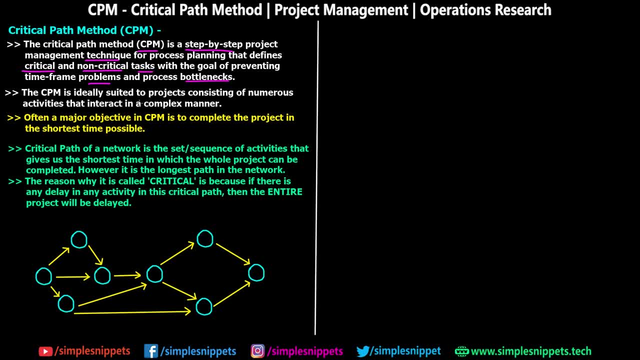 whenever you're going through a project. let's say, you are taking a construction project wherein you have to build a very huge building and it's a pretty complicated project, And so what happens is in such projects, there are certain tasks which are very critical. 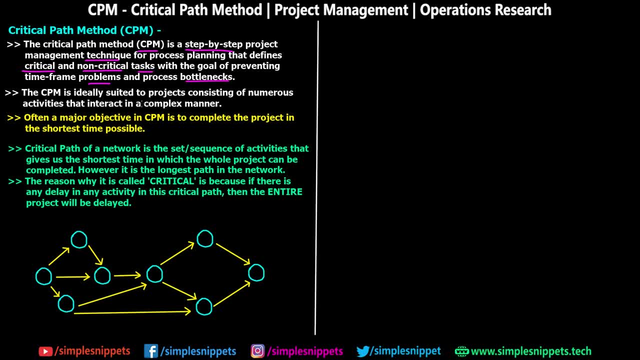 which means that if they get delayed, all the further tasks also get delayed and your entire project gets delayed. So those are some critical tasks And some some are non critical tasks, wherein you can delay the timeline for that task but the entire project timeline. 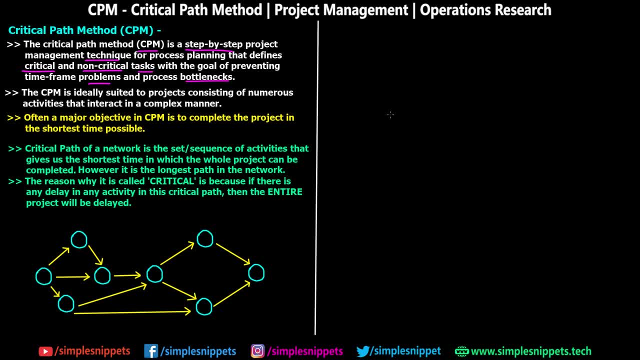 will not be delayed. So let's say, for example, in a construction business, if you are starting to develop a building, if you do not lay the foundation, then the first floor or the floors above can never be made. So the first floor or the floors above can never be made. And 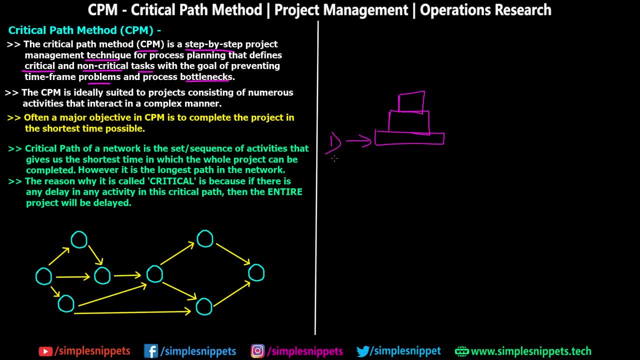 right. so as long as you keep delaying this first step, your second and third step will never happen and your entire project will also get delayed. so in this case, the laying of the foundation in the ground floor is one of the most critical activity in a construction right. so this was just a very 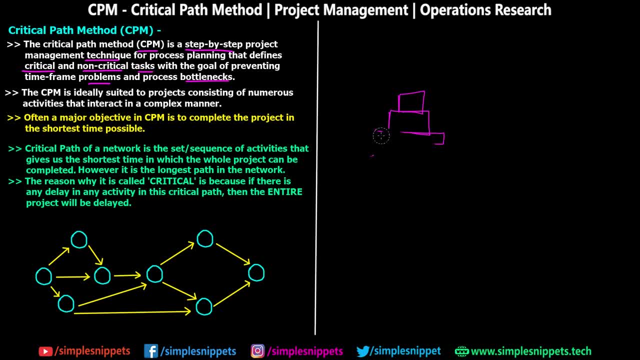 basic example. what happens is many a times in project management we do not understand what are the critical tasks and what are the tasks which can be delayed. so this cpm technique helps us understand which are the critical tasks and which are the non-critical tasks and, depending 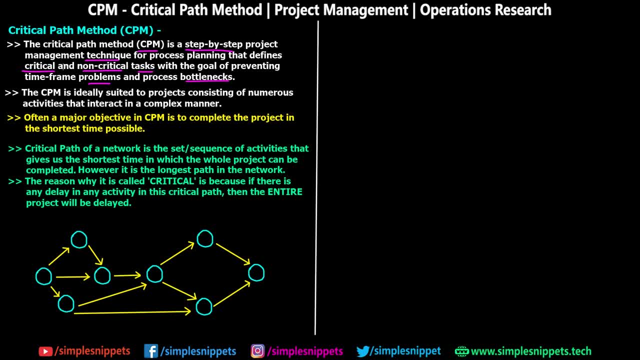 upon that you can allocate your resources and time to those tasks. so it is ideally suited for projects which consist of numerous activities and interact in a complex manner, and often a major objective in cpm is to complete the project in the shortest possible time. so, as i mentioned, 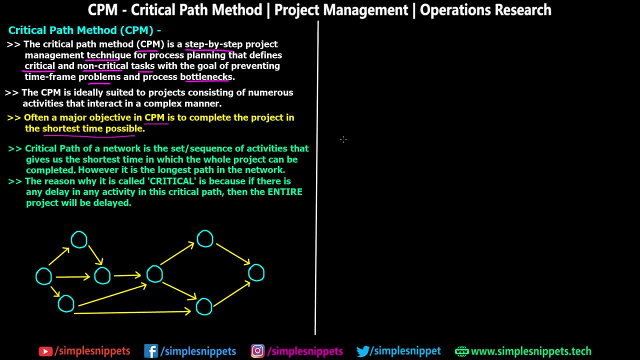 if the critical task is delayed, the entire project gets delayed, right? so our major goal most of the times using cpm is to reduce that time to the most shortest possible time. so what exactly is this critical path? so critical path of a network. so we've been drawing network diagrams, right? so network diagrams consist of set of activities and 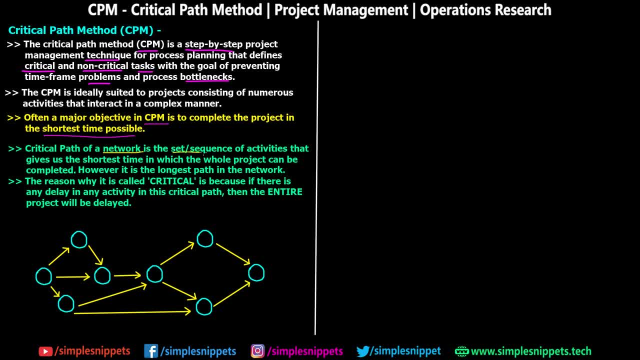 events. so, basically, critical path of a network is the set of activities that give us the shortest time in which the whole project can be completed. however, it is the longest path in the network, so this sounds contradictory, but what it is saying is: the critical path is the set of all. 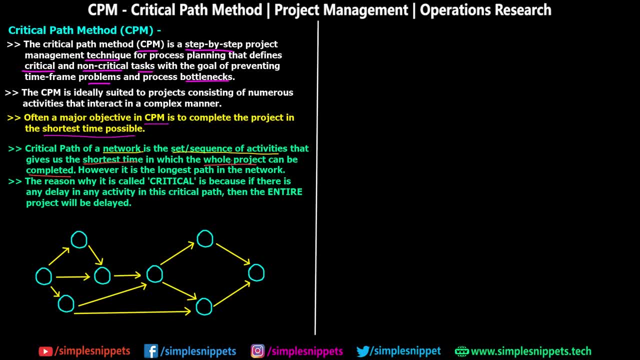 the activities that give us the shortest time in which the whole project can be done. so we know that. okay, this much is the minimum amount of time which will take, because all these activities are critical activities, so we have to make them or we have to complete them in exact. 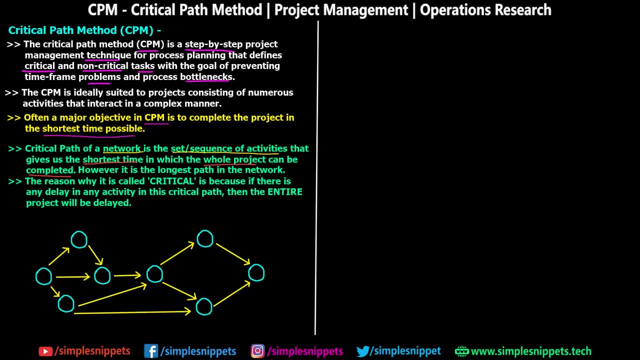 time so that the project doesn't get delayed. but basically it is the longest path in the network. so you'll find this out in the numerical when we go ahead and solve it. and the reason, as i mentioned, why it is called critical is because if there is delay in any activity, any one single activity, 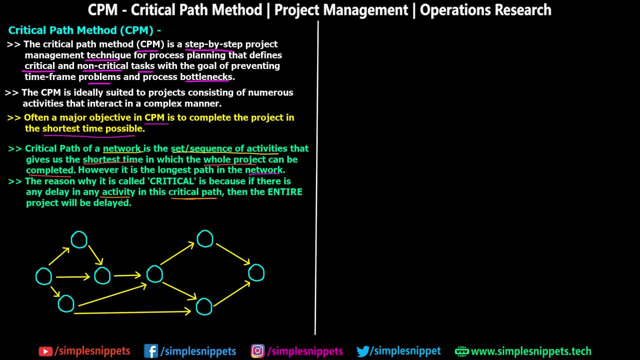 in the critical path, then the entire project will be delayed, so that's why it is called critical. so here we have a very basic network diagram, and what i'm trying to depict over here is, if this is starting, point a and this is ending, point b. so this is the first event and this is the last event. 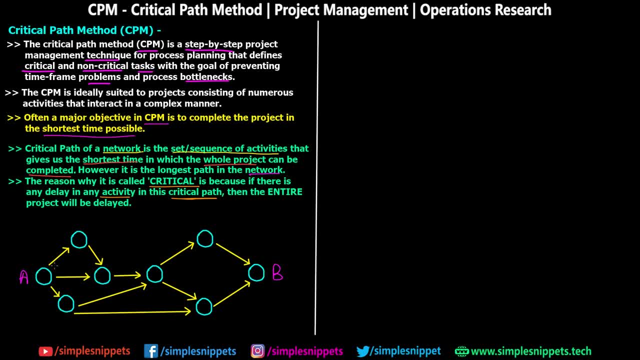 to reach from a to b. you can see that we have multiple paths, so we can go like this, we can go like this, then we can go from over here to here to here. so this is one path, right? another path would be starting from this event. go to this, go to this, so we didn't take this turn again. you can. 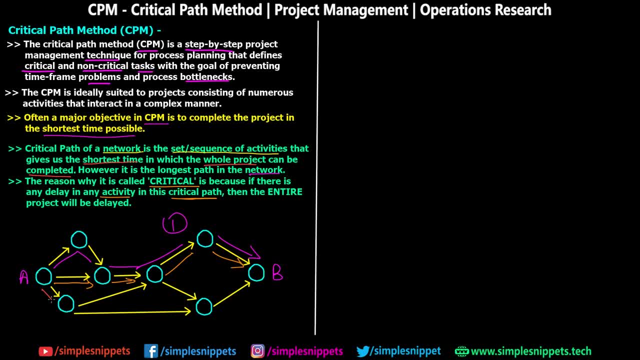 go up and go down. one more way is you can go down, go from this event to this event and then directly to the end. so you can see we have multiple paths in between, so not all of them are going to be critical paths. so these are the different paths which. 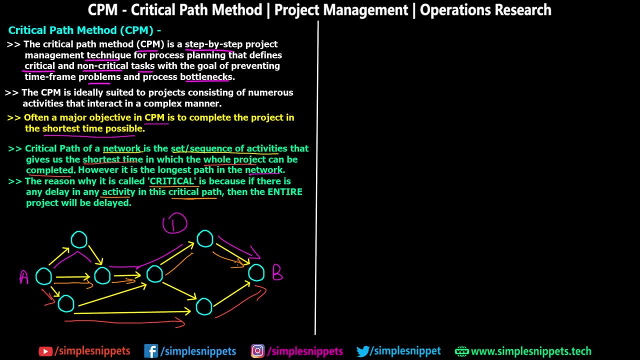 start from the starting event till the end event, and we only have to find out the critical path, which is the most important one. so this is what we are going to be finding out in this numerical, and this was a little bit of theory. now let's actually see a numerical based on critical path. okay, so, as 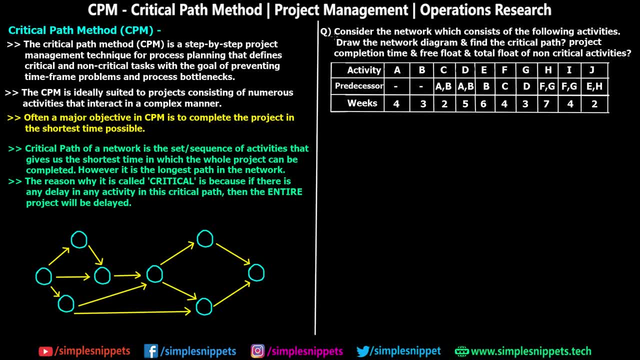 you can see on the screen, we have our question. let me just read it out quickly. consider the network. so we've been given a table with activities predecessors and one more extra column, which is the weeks column, or in this case it is rows. now we have to draw the network diagram and find 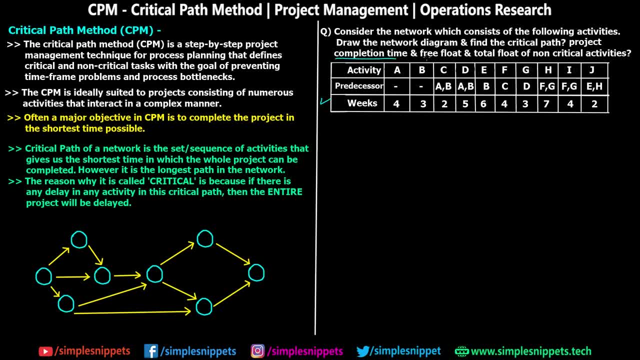 the critical path. we have to find the project completion time and we have to find free float and total float of the non-critical activities. so i'll explain what free float, total float is as we move ahead in this numerical, because this is something that is new and again we also have 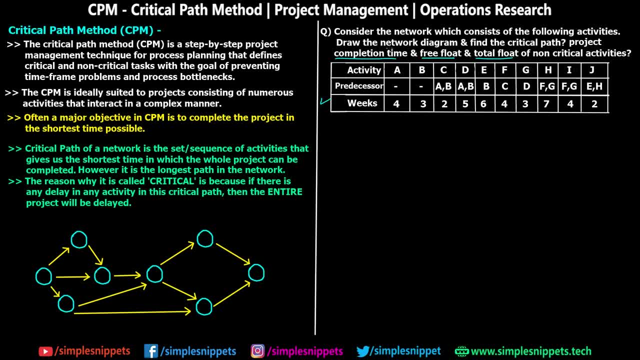 to find the critical path, which is also new. but we've already seen what is a network diagram. so in the previous couple of videos we've understood why we need to draw a network diagram and how it gives us an idea about the entire project development. so we'll 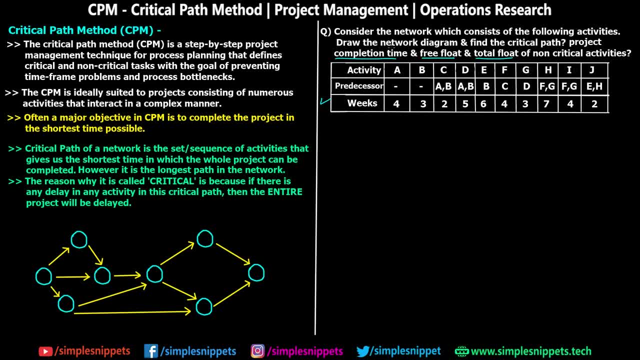 quickly draw this network diagram and not waste a lot of time on it, because we will have to calculate critical path, free flow, total float, so this will go a little bit lengthy otherwise. so let's start off with the drawing of network diagram. i hope you've already seen the previous two videos, because 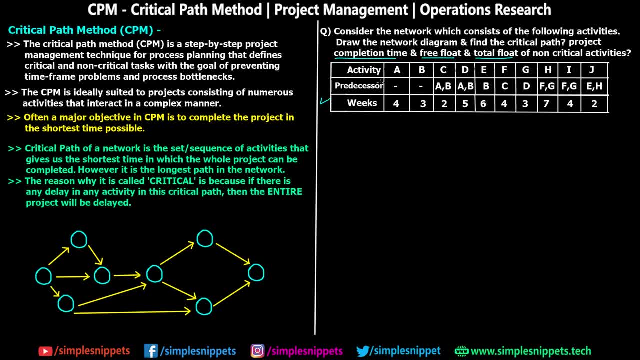 that's where we took different examples of network diagram and i hope you already know how to draw a network diagram, so let's quickly draw this rough network diagram. so, starting off with the first node, we have activity a and b, so there is no predecessor for a and b, so i'm gonna say this is: 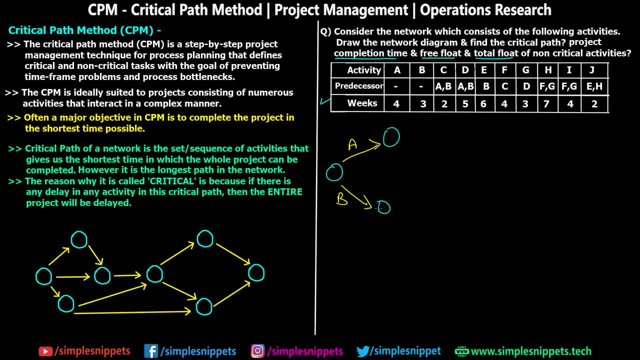 a and this is b, resulting in two different events. then we have c, which requires a and b, and we also have d, which requires a and b. so since these two are splitting to two different events, we have to join them with a dummy. we've talked about what is a dummy event in the previous video, so this is how. 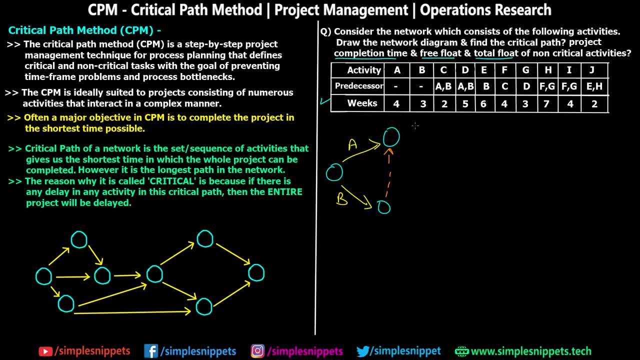 we join it and now c can be executed. so let's draw c activity, which will result in another event. so c is also initiated from this node itself or this event itself, because d also requires a and b to happen. so at this event a and b has already happened. so this is d. e requires b to happen. 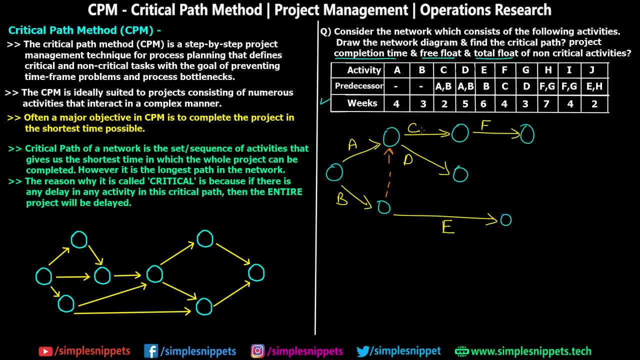 so we can draw e over here. f requires c to happen. c is happened over here, resulting in this event- and then f can happen. g requires d to happen, but h requires f and g to happen. so f and g needs to be combined. so i'm just going to combine this. so now h can happen. but before drawing h, you can see at: 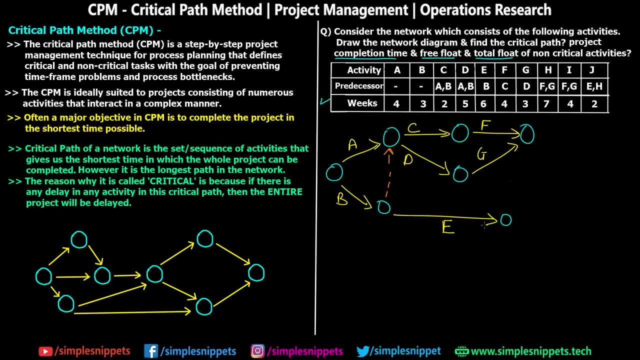 j activity. j activity requires e and h to happen. so e happened and resulted in this event. and what we can do is we can take this h activity and point it over here so that afterwards j can happen from this event. and i requires f and g to happen. so f and g happened over here and resulted in this. 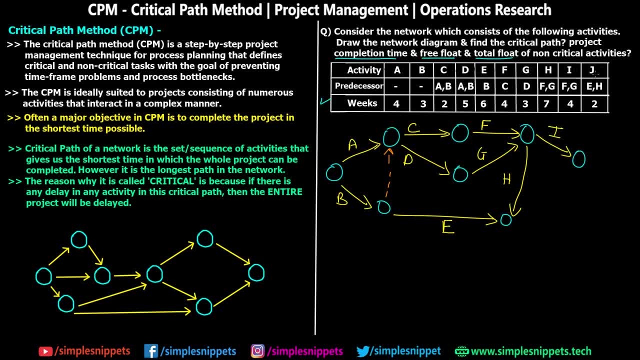 node or event, so we can draw i over here. and lastly, j will require e and h, so e and h meet at this point. and just to make this network diagram a closed network diagram, we can just connect this and name it as j. so yeah, this is the rough network diagram, but now you can see we also have 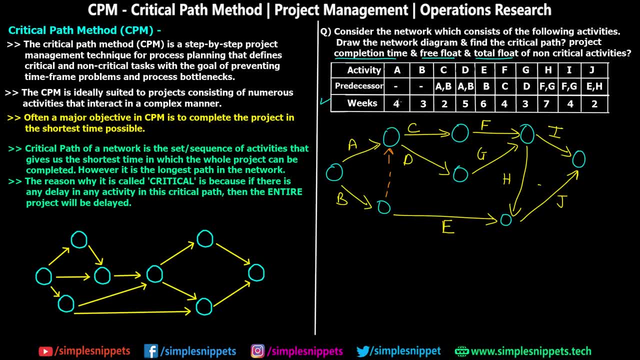 weeks associated with each activity. so what we have to do is we have to write down weeks along with the activities. so a requires four, b requires three, and this is in weeks. c requires two, so on and so forth. so what i'll do is i'll quickly erase this entire rough diagram that we 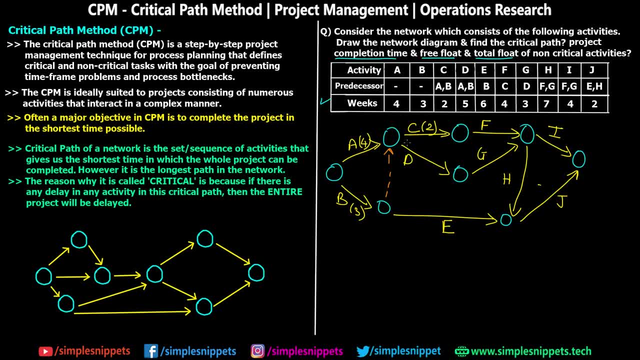 drew and i'll draw a proper diagram and then you can copy that diagram, because there are a few more things that we need to add into that diagram as well for calculating the cpm. that is the critical path. okay, so, as you can see on the screen, this is that same network diagram that. 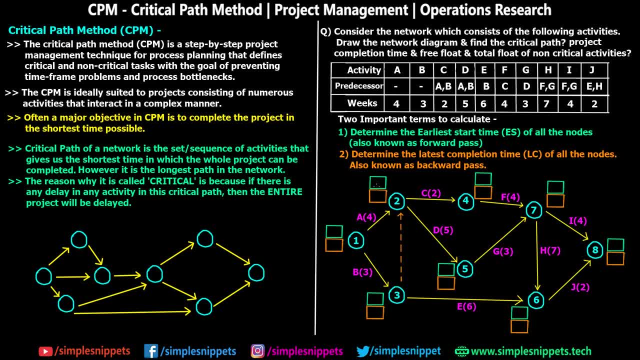 we drew in the rough, but i have certain things added over here, that is, these two boxes. otherwise the diagram is pretty much the same and i have also numbered the events. but you don't have to number it. i have written the weeks and the activity name in pink, so you can see activity a. 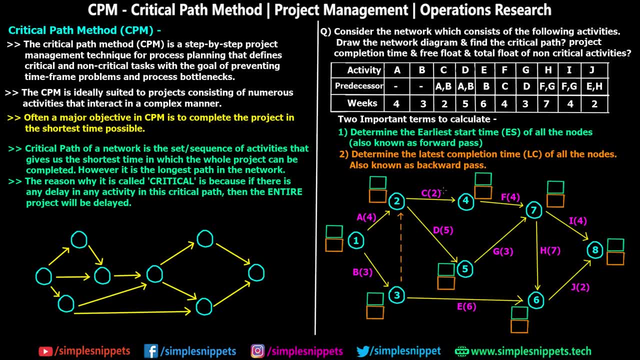 requires four weeks. so this is coming from over here, and all the other activities also. and now talking about these two boxes. so when we are supposed to calculate the critical path, we need to calculate the time, that we need to calculate the time for every activity or for every actual event. 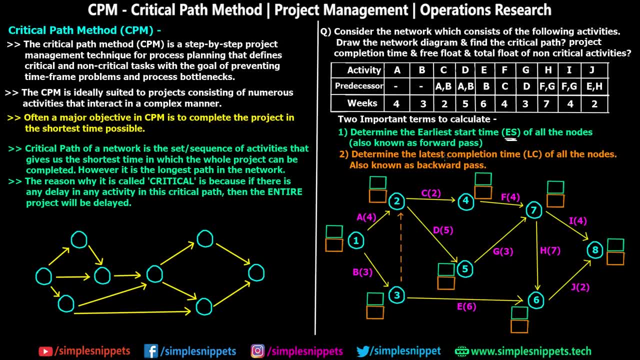 okay, so this is for these events, and these two things are known as earliest start time, which is denoted by es, and latest completion time, which is denoted by lc. so the green box is for early start, yes, and lc is for latest completion time for each of these events. so how do we go about? 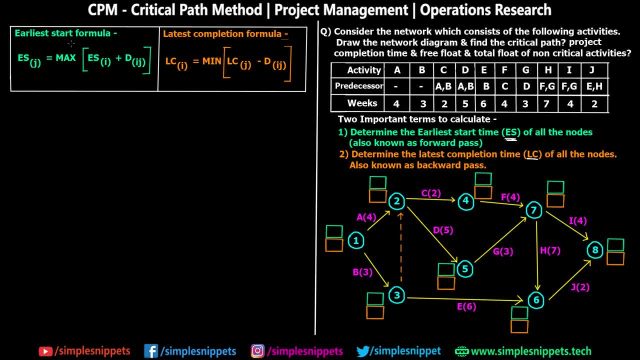 calculating these values. so let me just show you the formula first. okay, so, as you can see on the top left corner, these are the two formulas: earlier start formula and latest completion formula. so earliest start of j is equal to max of es, of i plus d of ij. now d is the distance which is 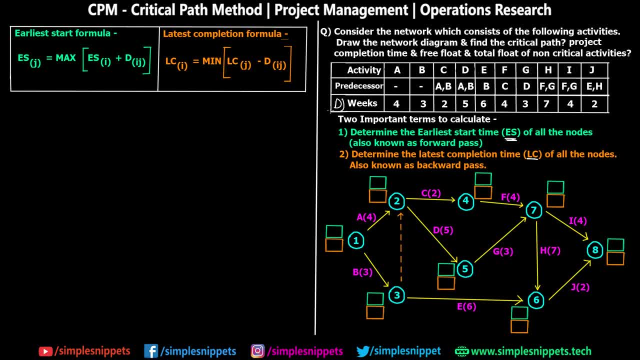 basically the weak value. so this is basically the d value always and latest completion time is given by lc of i, which is equal to minimum of lc of j minus d of ij. now, i know these formulas sound a little bit vague, but let's try to implement them in the numerical, so when you're 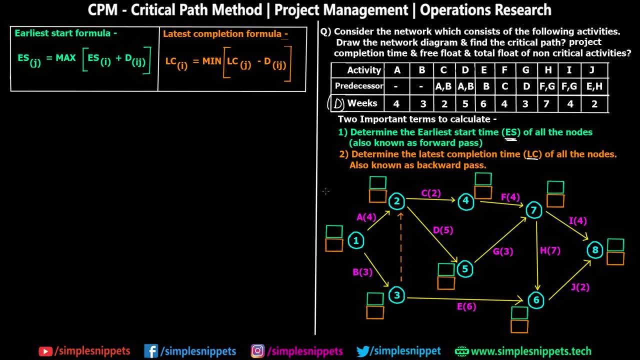 starting off with earliest start time. we have to start from left to right, that is, from the first event to the last event, so you have to go in this direction. okay, also for the first event, that is the number one event, the earliest start time is always going to be zero. so let me just write down: 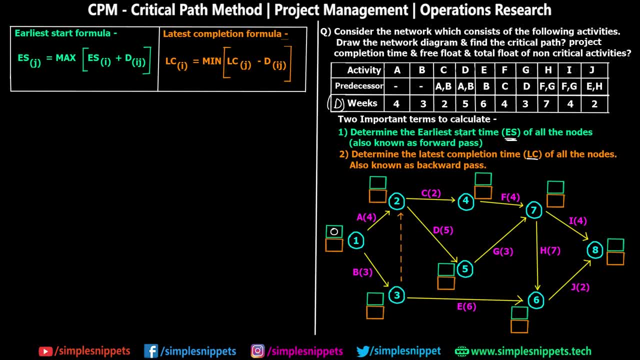 zero over here. so this is something that is by default happening, because earlier start time is basically how early can activity or an event start? okay, so you know, this is the first, very first event, so obviously there is nothing that it has to depend on, so this event can immediately start off. 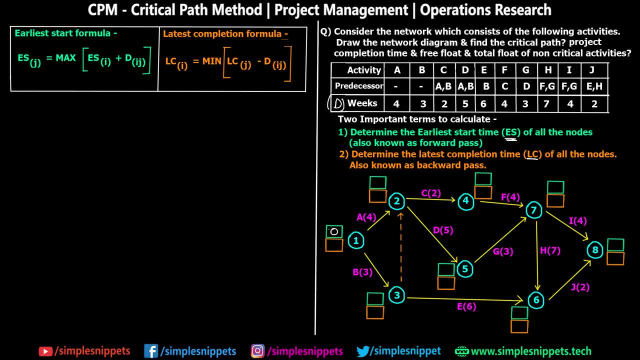 and this is in weeks, so it can start off in zeroth week itself, right? so that's why zero? now let's calculate earlier start time for this third node. now, as i mentioned, this numbering is not important. you can calculate for this or this. let's calculate for number three, so the formula is earliest start. 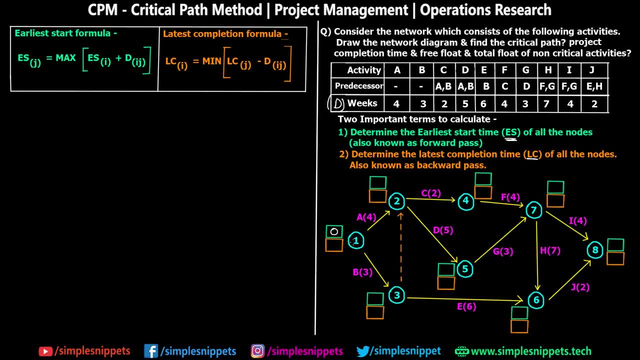 time of j. now we have two events in this case, that is, we are going from one to three right, so event one to event three. this is what is happening. so when i see es of j, it means that i'm referring to this value. that is the second event that i'm moving on to, because we are moving on from one to three right. 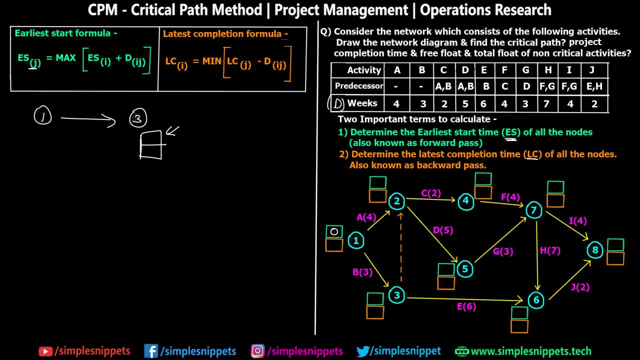 so es of j means es of the second event. so this is given by max of es of i. so es of i is the es value of the first event, which we just calculated as zero, okay, plus d of ij. so d of ij, as i mentioned, is the distance in weeks which is given as three. 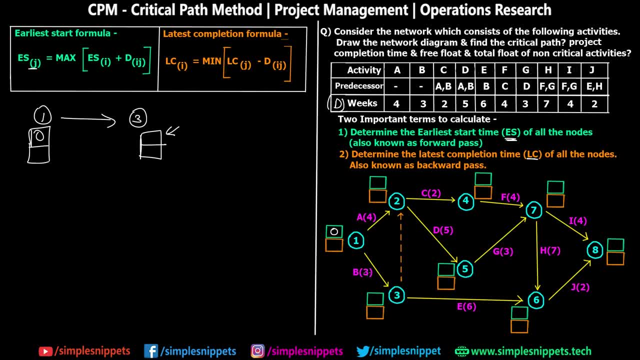 over here, right? so for the activity b, it requires three weeks. so we have to add this, so we have to take zero, which is es of i, that is early start of the first event, which is zero plus three, and this will give you four. now this max is used only when there are multiple activities coming in at a single node. 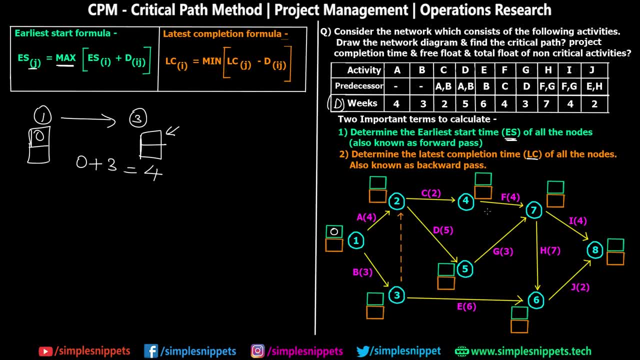 okay. so that situation will come as we move ahead in this numerical. so this would be zero plus three. so zero is es of i, that is, es of first event, and three is the distance, or three is the number of weeks required for activity b. so zero plus three is gonna be three. 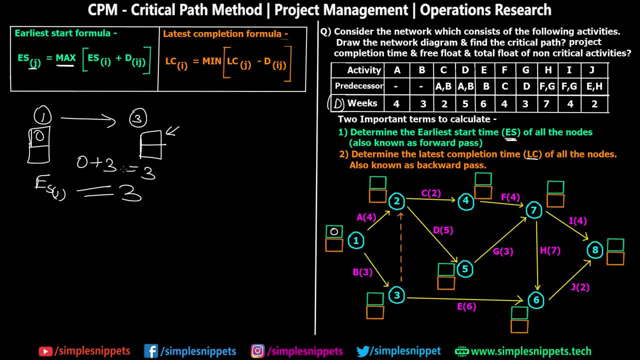 so this is: es of j is equal to three. okay, so i'm gonna write three over here. i hope you're getting this now if you are wondering what this max is used for. so max is used when multiple activities come at a single event. so that is when we have to compare the values of es of i plus. 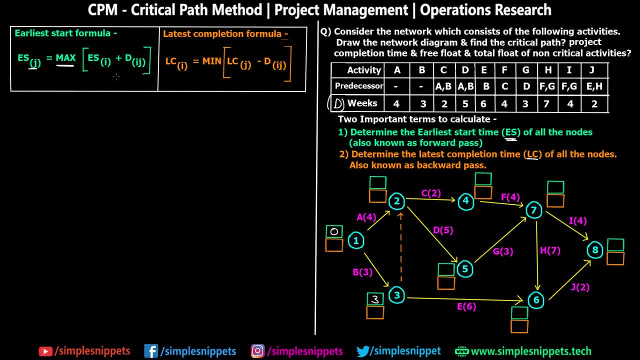 d of ij and take the maximum value. so we'll see that when we move ahead in this numerical, right now the max value is not needed. so similarly, let's calculate for event two. so for event two again, we have to use the same formula es of i. so for this we are going from 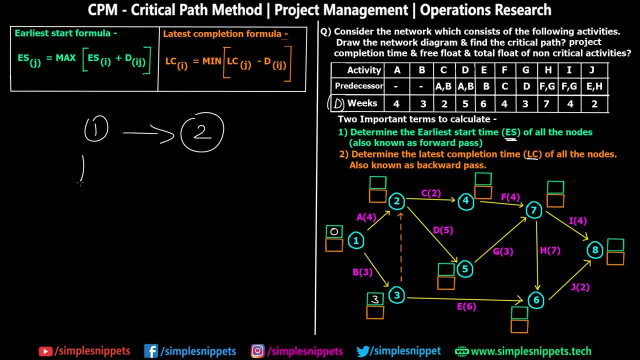 one to two, right? so es of i is going to be zero. so this is es of i and what we are calculating is es of j, right? this is the formula. we are calculating early start for event two. we've already calculated it for event one. we are calculating it for event two. it is given by: 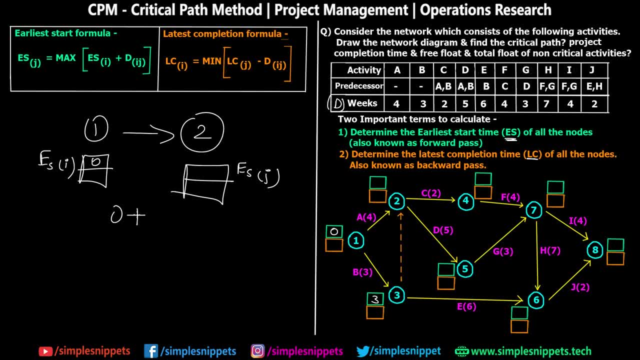 earliest start of the previous event. that is, this zero plus distance between the two events, which is, so this is going to be four, so i'm going to write four over here. that is, i'm going to write four over here, so i hope you're getting how to calculate early start. now let's speed up and 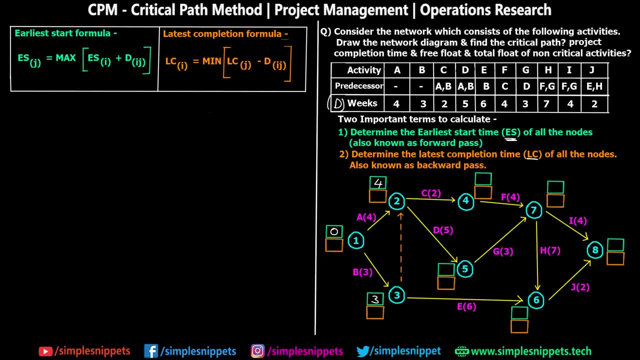 calculate early start for other events as well. so let's take a look at this event five. so early start of event five would be early start of the previous event, which is two. so we came from two to five. right, we are moving from left to right, so from two to five, the early start of two is four. 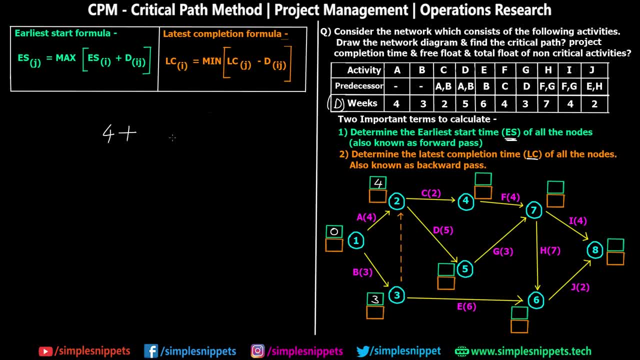 that is, es of i in this case is four plus the distance between them is five. so this is four plus five, which is going to be 9. so I'm going to write 9 over here for this event. 4: we came from 2 to 4. 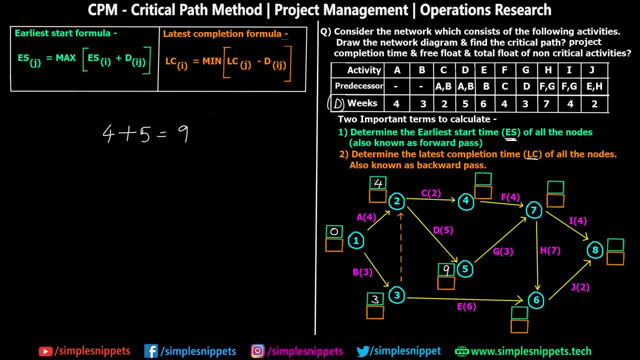 so early start of 4 is going to be early start of 2. that is 4 plus the distance between them, which is 2, which is going to be 6. so I'm going to write 6 over here for event 6. you can see that there are. 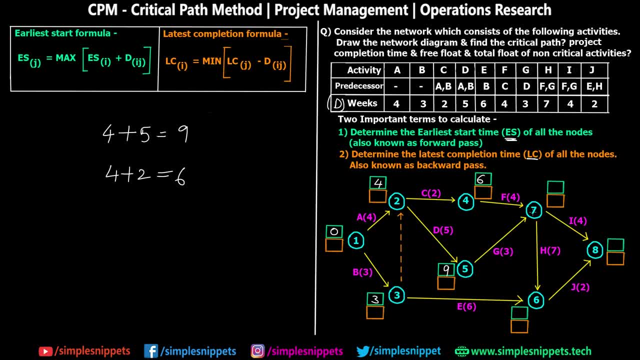 two arrows coming in, so we first have to calculate value of event 7. first, because we've calculated the value of early start for event 4 and event 5, so in this case we are going to be using the maximum function. so let's calculate es value when you come from event 4 to event 7. so when you come, 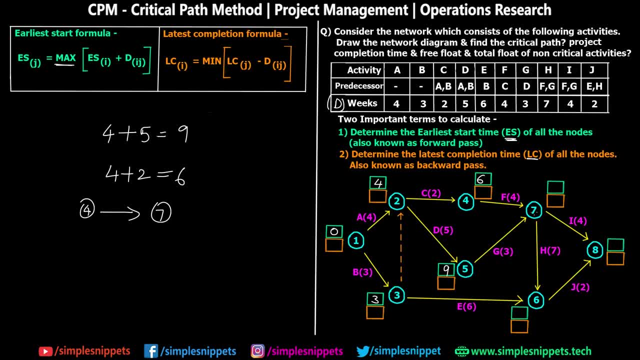 from 4 to 7. the es value of 7, that is, es of j, is going to be early start of event. 4, which is 6. this is that value plus d of ij. that is distance between them, which is 4. so this is going to be 10. 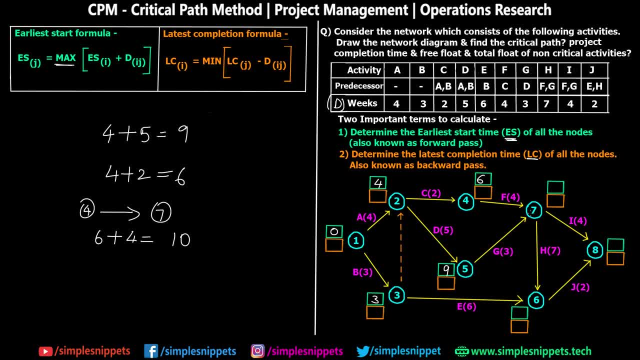 however, you can see there is one more activity which is coming in to the seventh event. so there are two options now. so we can come from 4 to 7 also and 5 to 7 also. so let's calculate es of 7 when you come from 5 to 7. so when you come from 5 to 7, that is 5 to 7, you can. 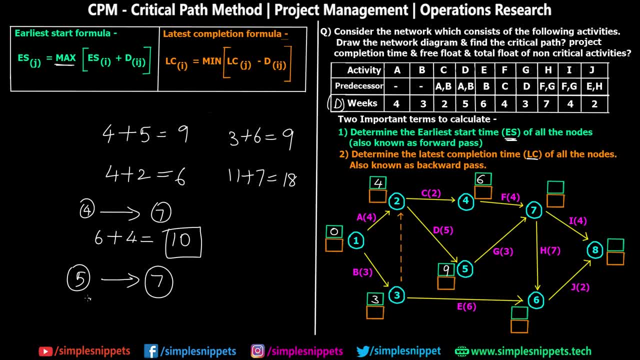 see that the es value of 5 is 9, so we have 9, plus the distance between 5 and 7 is 3, so this is going to give you 12.. so now you can see we have two different options. that is coming from 4 to 7. we. 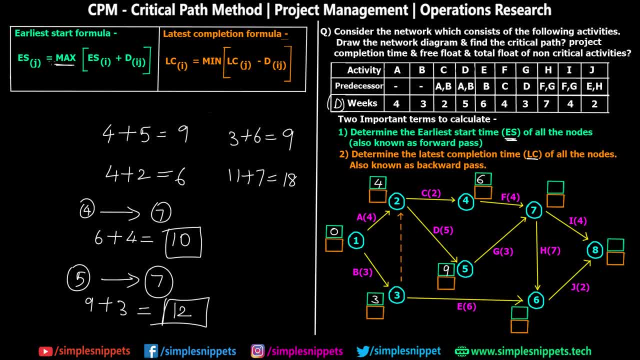 have 10, and coming from 5 to 7, we have 12.. so this is where the max function comes into picture and we have to take the maximum out of the two, which is 12.. so I'm going to write 12 over here. 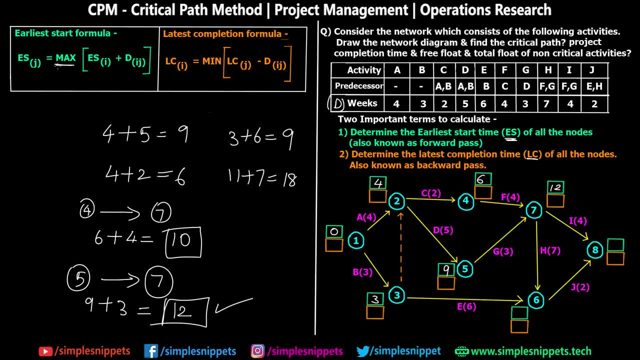 so I hope you are getting where you have to use maximum. we have to use maximum only when multiple activities are coming in at the same event. okay, so now we can easily calculate the same thing for event 6, because we can come from 7 to 6 and we can come from 3 to 6, so when we come from 3 to 6, 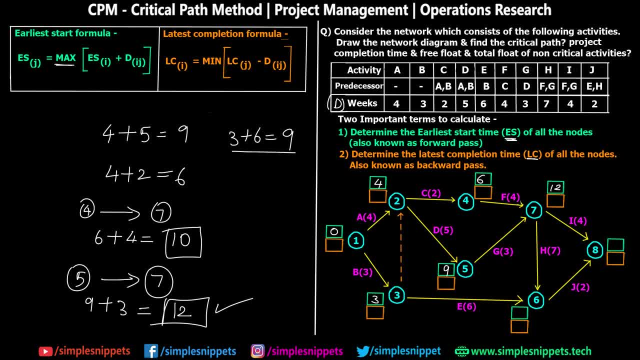 we have 3 plus 6, which is 9, over here. similarly, when we come from 7 to 6, we have 12 plus 7, which is going to be 19. so obviously we are going to select 19, because 19 is greater than 9 and for 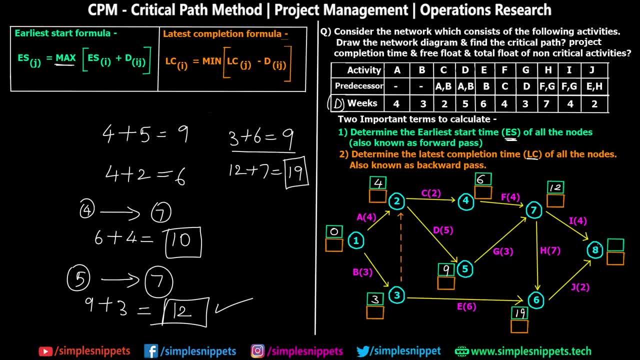 example, we have two options: we can come from 7 to 8 or we can come from 6 to 8. so when we come from 7 to 8, we have 12 plus 4, which is 16. so 12 plus 4, which is 16. and when we come from 6 to 8, we have 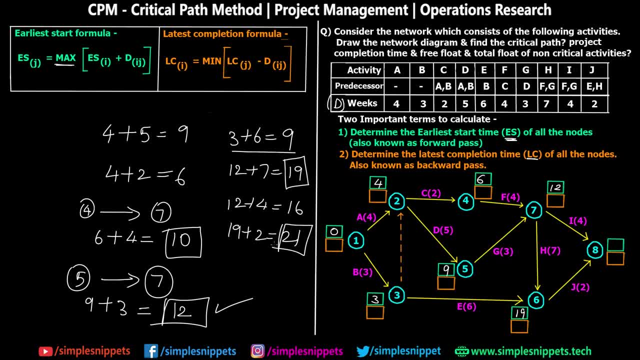 19 plus 2, which is 21, and obviously we're going to select 21 because we have to select the maximum one, so I'm going to write 21 over here. okay, so we've calculated all the earliest start times by using this formula and I hope you've got a very good understanding of how to go about calculating this. 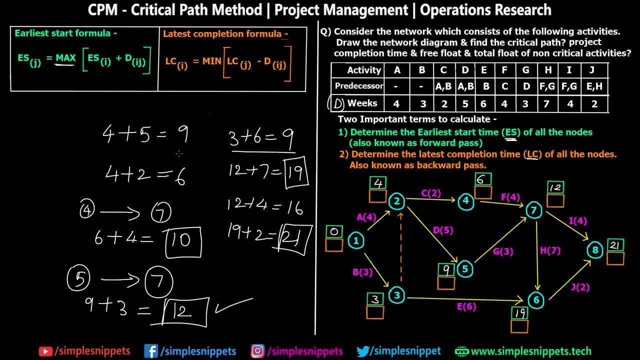 we went a little bit slow because this was a formula which is going to give you the maximum first time, but I hope you've understood this. so now we have to calculate latest completion time, and for latest completion time we have to go from right to left in this direction. so we have to start. 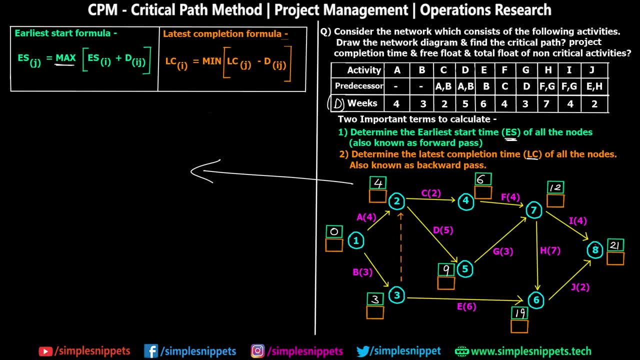 from the last event and we have to come to the first event, and for the last event, the latest completion time is always going to be equal to the earliest start time, so it's going to be 21 over here, so this is something that is by default happening, and now we have to go backwards, okay? 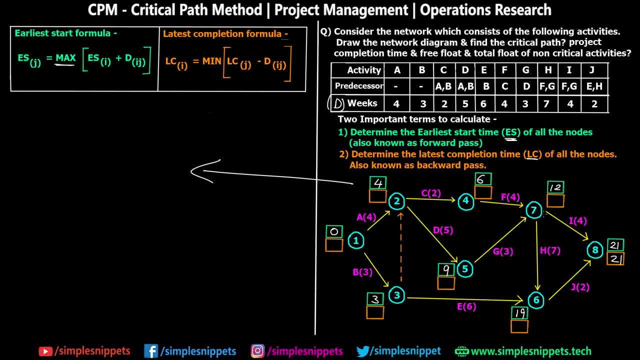 and the same concept applies when there are multiple activities starting from an event. we have to use the concept of minimum. so here we have to use minimum and we have to do subtraction instead of addition. okay, so first you can see, we can go from 8 to 6, because from 6 only 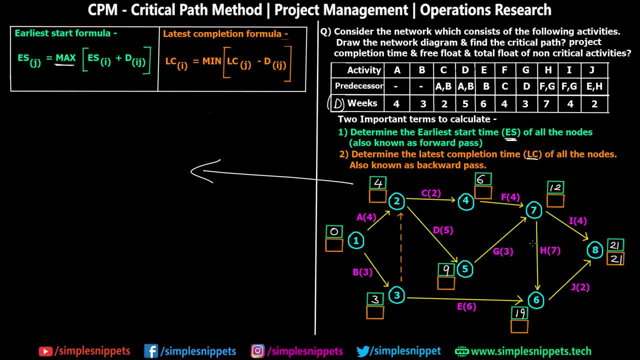 one activity is starting. you can see, from 7 we have two activities starting. so first we have to calculate latest completion time for 6. so how do we go about this? so lc of i now, in this case, when we are going backwards, that is when we are going from 6 to 8, that is, we are basically going backwards. 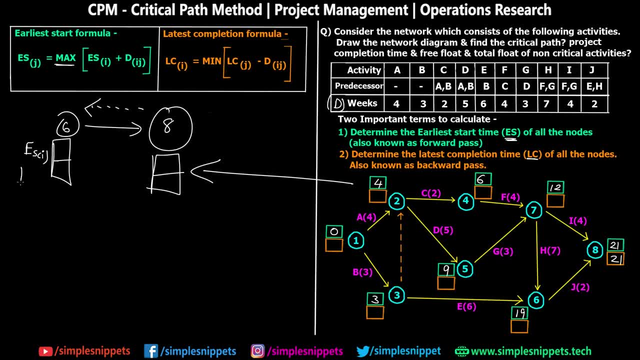 so in this case, this is going to be es of i and this is going to be lc of i and again this is going to be lc of j. okay, so here what we are doing is we are calculating lc of i, that is lc of previous event. right, we are calculating lc for 6th event and not the 8th event, so this is the previous. 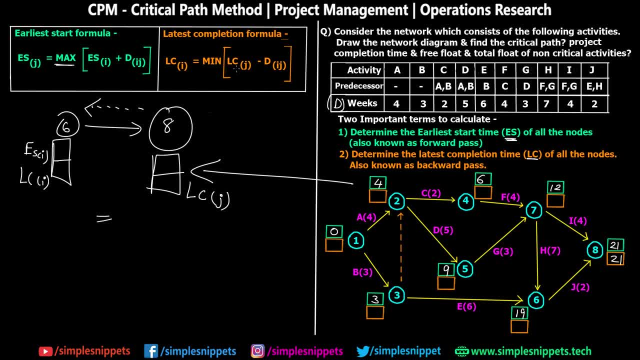 event. so lc of i is given by minimum of lc of j. so lc of j is lc value of the next activity. so we've already calculated it as 21. so 21 minus the distance from the next activity to the next activity is the distance between the two events, which is 2 over here right. so 21 minus 2 is going to give you. 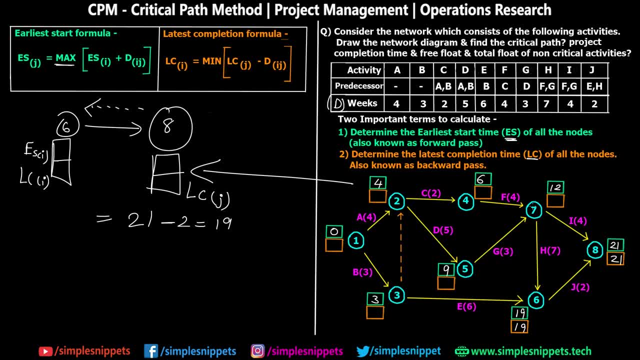 19. so this is what i'm going to write over here. now let's calculate the lc value for 7th event. so for 7th event you can see there are two activities starting from 7th event. so when we go back also, we have two different options. right, we can go back from 6 to 7 or we can go back from. 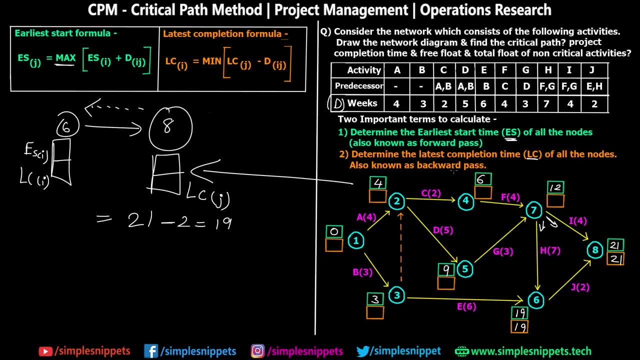 8 to 7. so this is where that minimum concept is going to be applied. so let's first calculate when we go back from 8 to 7. so when we go back from 8 to 7, the formula is lc of j. that is the minimum. 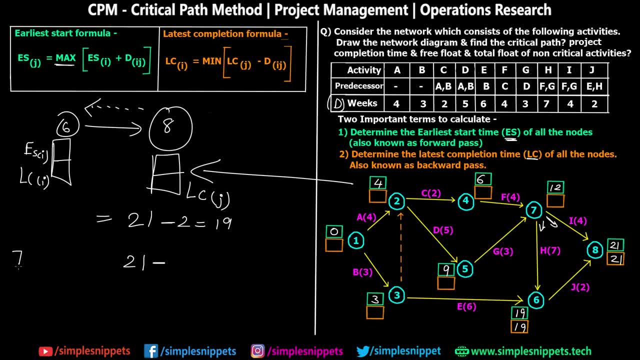 that is 21, so let me just first write it down. when we go from 7 to 8, so for this we have 21 minus that is, 21 is lc value of 8 minus the distance, which is 4, so this is going to be 17. and when we 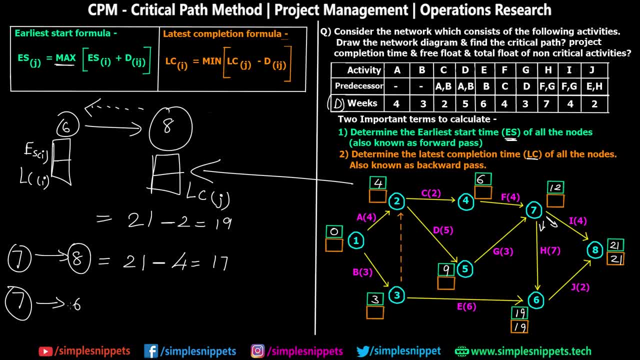 go from 6 to 7, so i'm writing it in reverse order. over here we have 19, which is because we are going in reverse order like this, right? so lc of j over here is 19 minus the distance is 7, so this is. 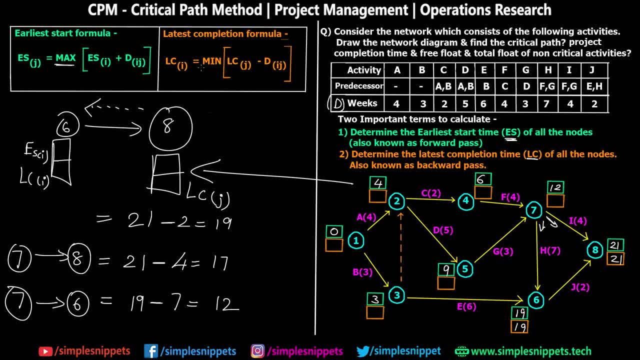 going to give us 12.. now we can't select maximum because in the formula we have to select minimum. so minimum out of 17 and 12 is 12, right? so this is why we are going to be selecting 12 over here. so i hope you are. 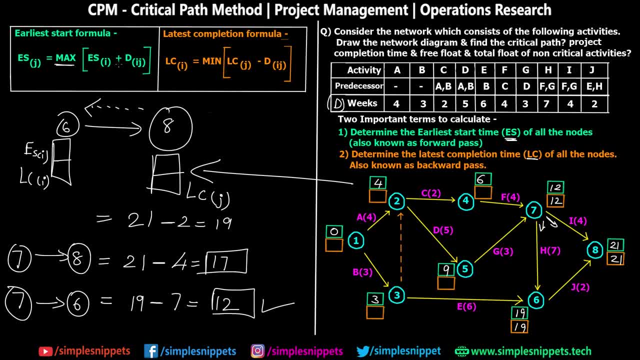 getting the difference between the two formulas. in one case, we are selecting maximum and there is addition. in other case, we are selecting minimum and there is subtraction. so now let's calculate the same thing for 4. let's do it a little faster, so from 7 to 4, when we are going. 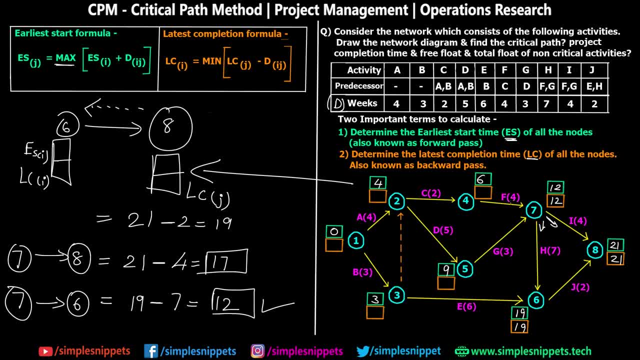 we have to take lc of j, that is 12 minus the distance, which is 4, and since there is no other arrow coming from this event, you only have one option, so no concept of minimum over here. so 12 minus 4 is directly going to give you 8. let's calculate that same thing for event 5, when you 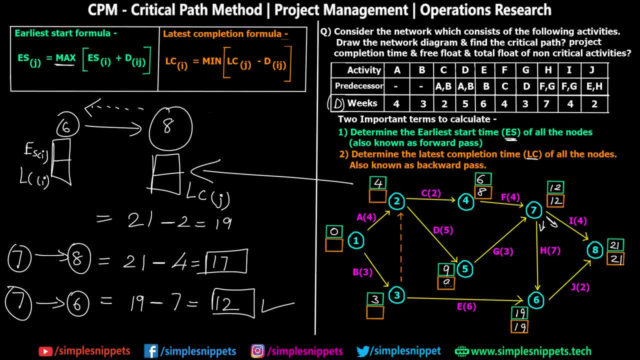 come from 7 to 5. we have 12 minus 3, which is 9, no other arrow coming from 5 or going from 5 to some other event. so no other two options. so for event 2 we have two options: we can come from 5. 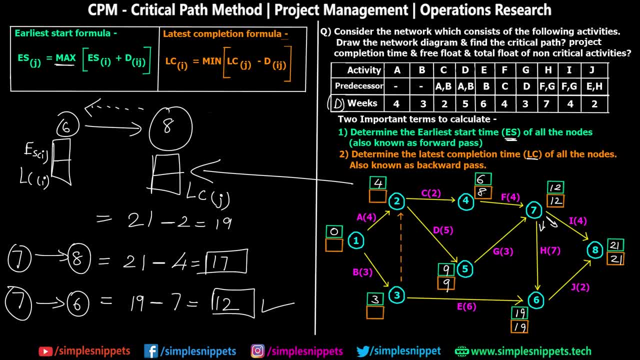 to 2, or we can come from 4 to 2. so when you come from 4 to 2, we have 8 minus 2, which is 6. so 8 is 4 minus the distance, that is 2, so we have 6 over here. and when you come from 5 to 2, we have 9. 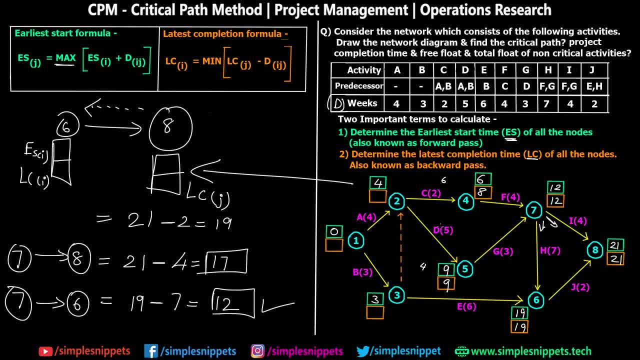 minus 5, which is 4, right, 9 is lc value of 5 and the distance is 5. so 9 minus 5 is going to give you 4. so out of 4 and 6, we know the minimum is 4, so i'm going to write 4 over here. lastly, coming 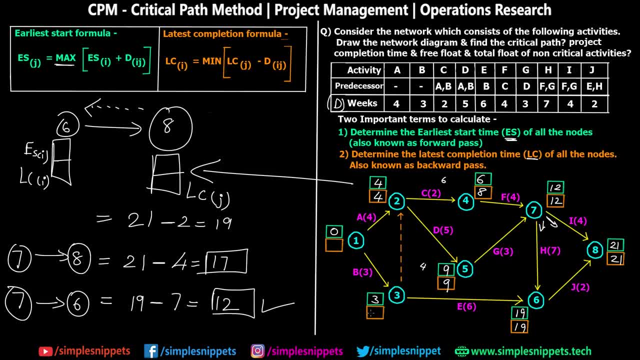 from 6 to 3, we have 19 minus 6, which is going to give you 13, and for the very first event, you can see we have two options: we can come from 2 to 1, or we can come from 6 to 3 and we can come from. 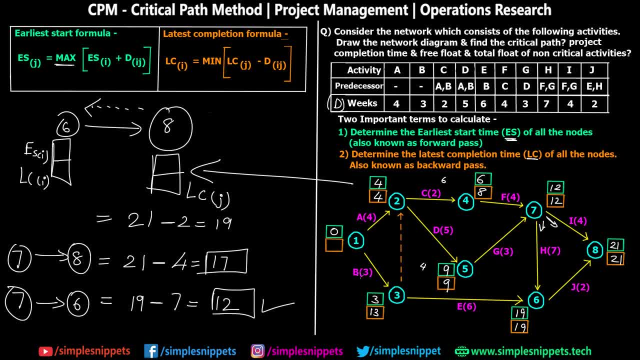 3 to 1. so when you come from 3 to 1, we have 13 minus 3, which is 10. when you come from 2 to 1, we have 4 minus 4, which is 0, and obviously we're going to select a small value. so this is 0. so 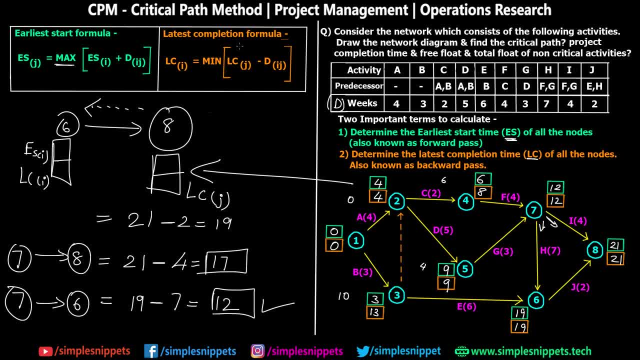 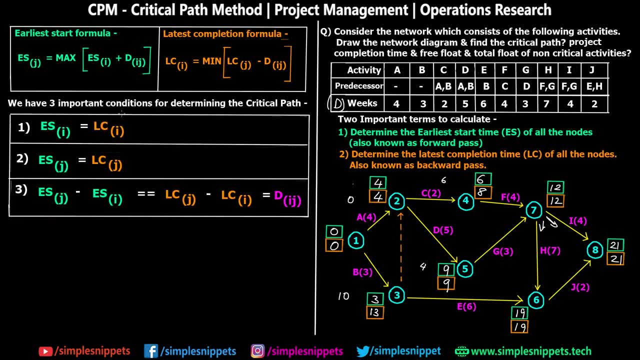 yeah, this was the calculation of early start and latest completion for all the events, and now we have to find out the critical path. so let's see how to go about calculating the critical path. so to calculate the critical path, we have three important conditions for determining whether it is a critical path or not. so we have: es of i is equal to lc. 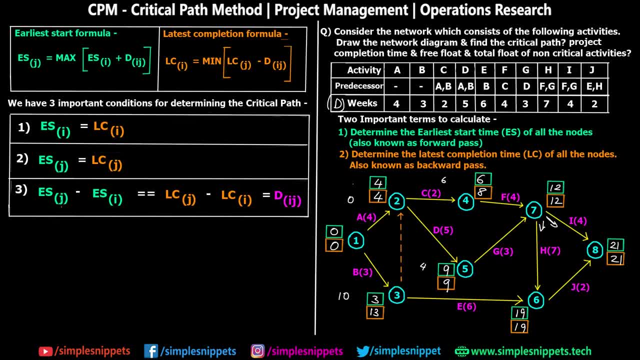 of i, es of j is equal to lc of j and es of j minus es of i is equal to lc of j minus lc of i, which is equal to the distance. so all of these need to be true. so basically, you cannot say that if this is true and this is false, then it is still a critical path. all of them have to be compulsorily. 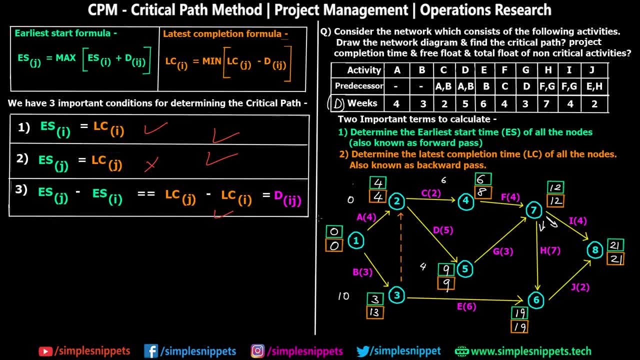 true for that part to be a critical path, but a very easy understanding of these three conditions is that wherever there is es equal to lc between the two events, that is a critical path. okay, so for example, you can see from event one and two, es and lc, es and lc, both are equal, so this. 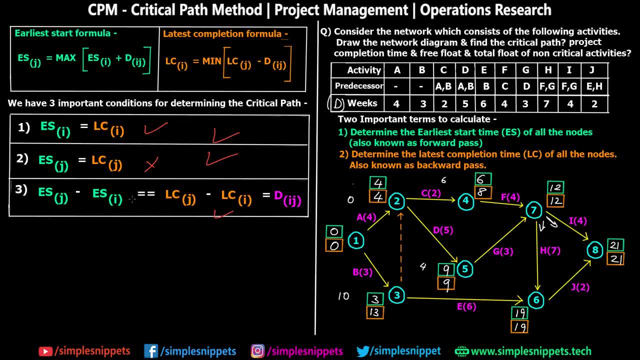 is a critical path. so that's the basic understanding of all these three conditions. so how do we mark this critical path? so let's mark this with red. so from one to two is a critical path and we have to go all the way till the last event, like this. so if you see, from two to four it is not a critical path. 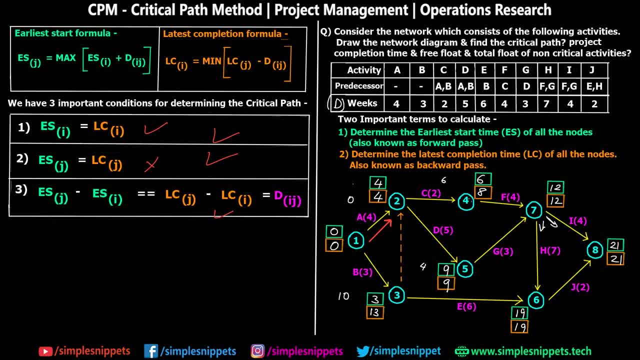 because for two, four and four is equal, that is, es and lc. but for the fourth event you can see six and eight. it's not equal. so this is not a critical path. so from two to four it is not a critical path, but if you see from two, 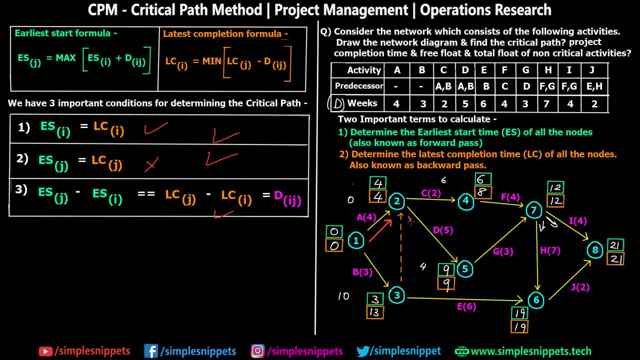 to five, you can see both es and lc. es and lc are same, so this is a critical path. from five to seven is a critical path, because both es and lc of five and seven are equal. from seven to twenty one is also a critical path. okay, so this is one critical path, starting from first event till the last. 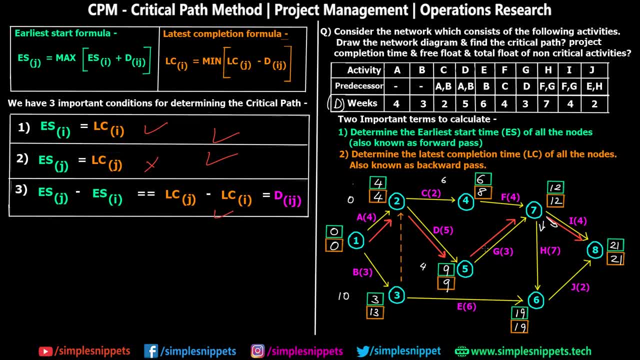 but now you can see, in this entire numerical we also have another critical path. so from 1 to 2, 2 to 5, 5 to 7, but you can also see from 7 to 6 is also a critical path, because es and lc of 7 and es and 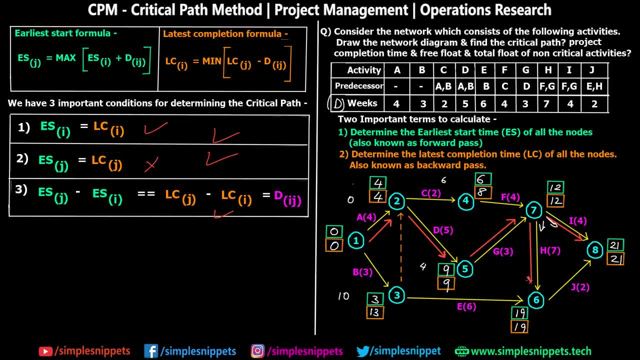 lc of 6 is also equal, so you can go from 7 to 6 also. so this is another critical path. and then you can go from 6 to 8, because from 6 to 8 is also a critical path, because both these values are same. 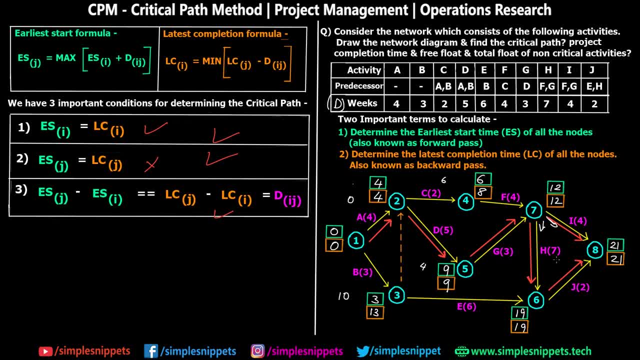 so in this specific numerical, we have two critical paths and let me just list them down as a final answer. so this is how the final answer should be like and if you're wondering why there is only one critical path, so remember, the definition of critical path is the. critical path is the. 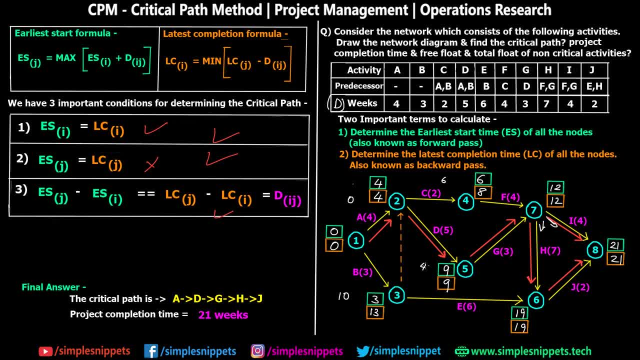 longest path in the entire project, right? so we have found out two critical paths. so the first path is from activity a to activity d to activity g to activity i. okay, so we go like this, like this, like this, and we reach the end. so what we have to do is we have to take the total of the weeks. 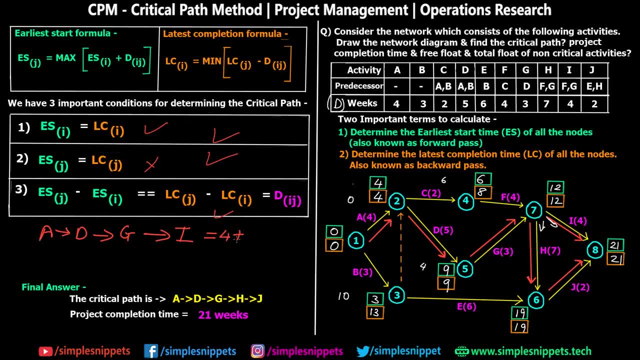 of these activities. so for a we took four weeks. for d we required five weeks. so we have to take the total of the weeks of these activities. so for a, we took four weeks. for g we required three and for the last one, that is, i, we required four. so this total comes down to: 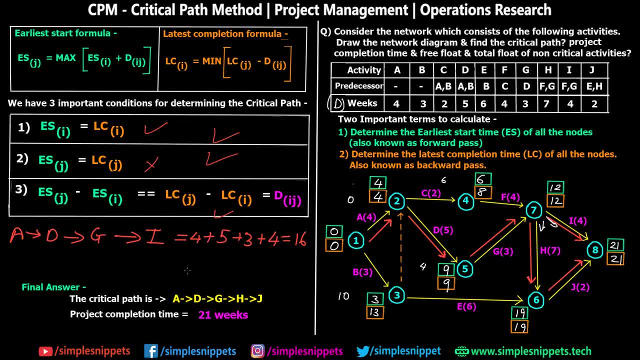 16, right? so this was one critical path. however, you can see that there is another critical path, which is from a to d, then d to g, then we have g to h and from h to j, so in that case, the total is coming down to 21. so if you add all of this, that is, 4 plus 5 plus 3 plus 7 plus 2- this will give you 21. 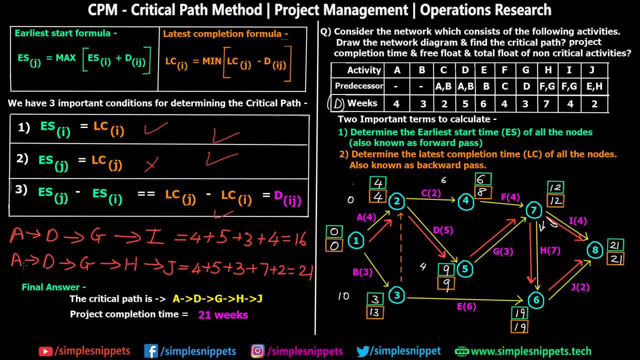 so 21 is larger than 16, so that is why the final critical path is this: a, d, g, h and g activities. okay, so this is the critical path and the project completion time is 21 weeks. so we've answered two questions out of the four questions, that is, we've calculated or found the critical path. 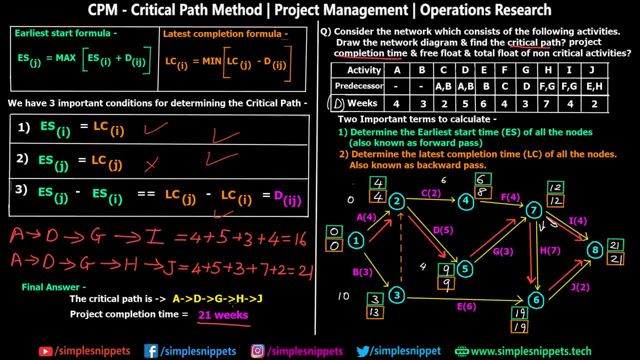 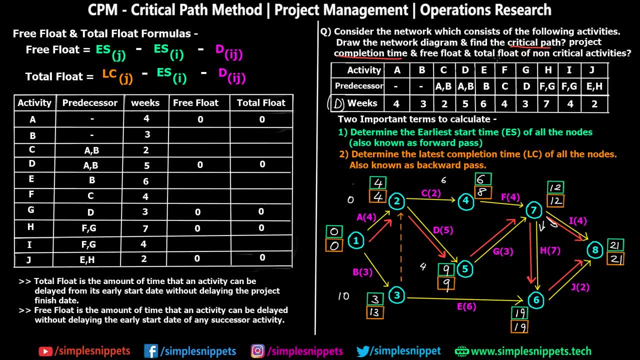 and we've also seen the project completion time, which is 21 weeks. so now we are left with free float and total float. so let's see what these things are. so in the question, what is asked is: we have to find out the free float and total float of the 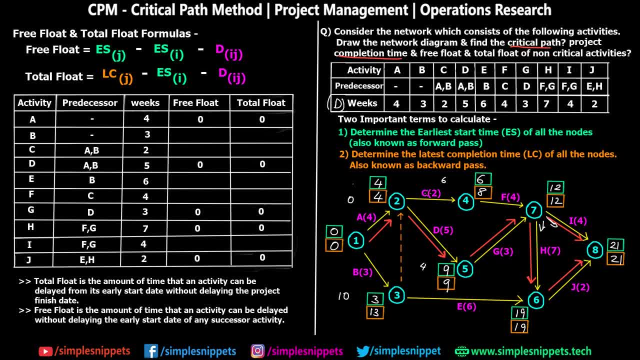 non-critical activities. okay, so we've already identified the critical activities, so i've redrawn this entire table and i have added two more columns, that is, free float and total float, and out of this we know the critical activities are a. we know the critical activity is d. 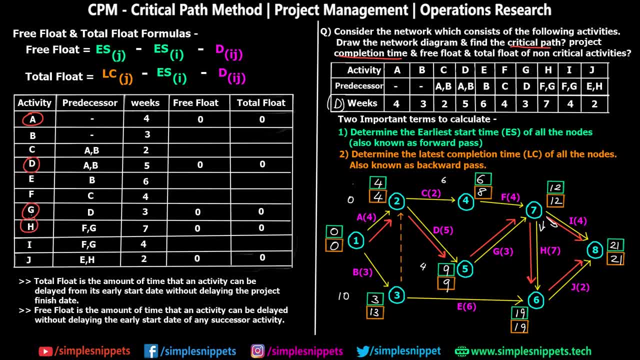 so we have a, we have d, we have g, we have h. that is, we have g, we have h and we have j. okay, so when it comes to free float and total float for these critical activities, that is, the activities which are on the critical path, the free float and total. 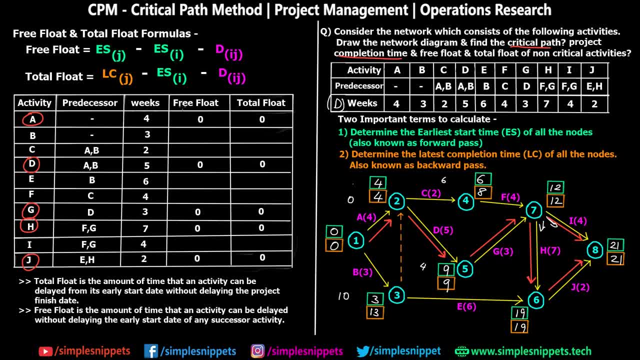 float for them is always going to be zero. so if you are wondering what is free float and total float? total float is the amount of time that an activity can be delayed from its early start date without delaying the project finish date, and free float is the amount of time that an activity can be. 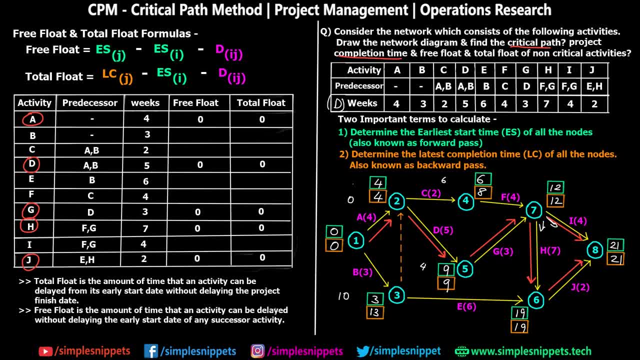 delayed without delaying the early start date of any successor activity. so take a moment and read this if you want to understand theoretically what it means. but that's not the focus of this numerical right now. essentially, all the activities on the critical path can never be delayed because if they 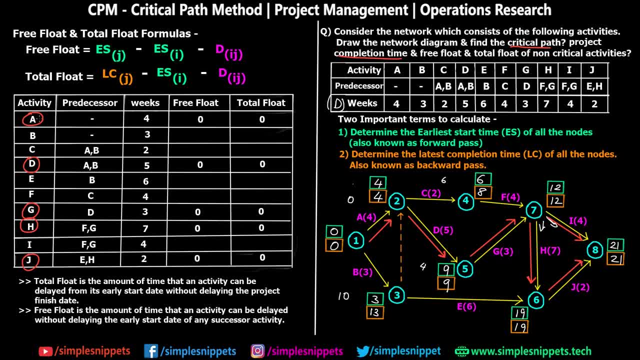 get even delayed by one week or any amount, the entire project will get delayed. so that is the basic definition of critical path, right? all the activities on the critical path have to be finished in their respective times. so that's why they have zero free float and zero total float, so we only 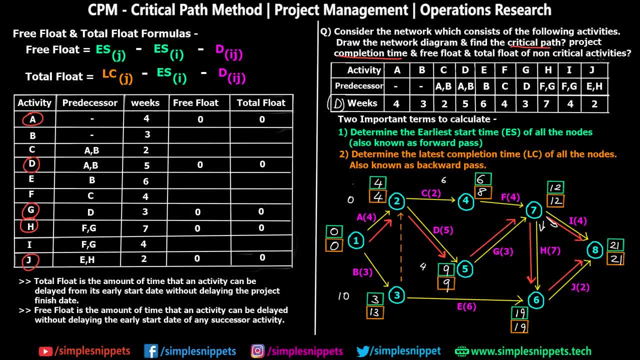 have to find out free float and total float for non-critical activities. so to do that we have again two formulas. so make a note of these formulas. so for free float, we have es of j minus es of i minus the distance between the two. for total float, we have lc of j. 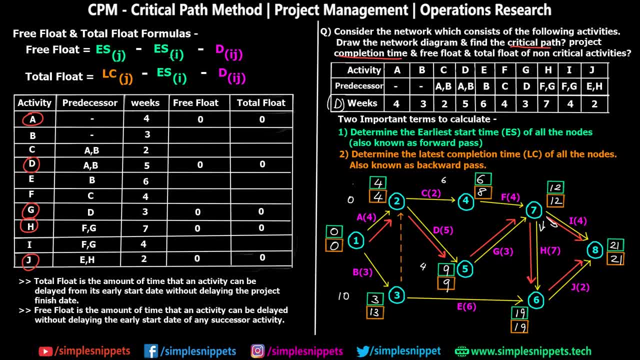 minus es of i, minus the distance between the two. so using these formulas- and already we've calculated es and lc values for all the events- let's quickly calculate the free float and total float for all the non-critical activities. so for b, if you observe, for this b activity, 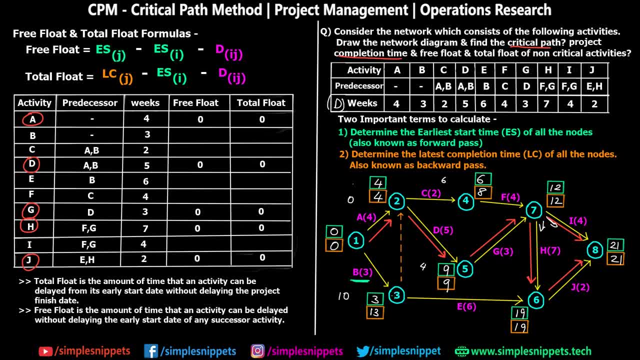 these two events are involved. that is event number one to three. so in this case es of j is the next event, so early start is three. so we have three minus early start of previous event. so for one and previous event is one and early start of one is zero minus the distance between them. so the distance 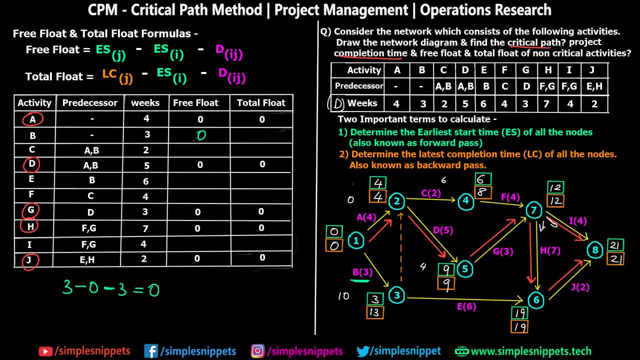 is three. so this is going to give you zero. so i'm going to write zero over here. similarly, the total float is going to be lc of j. so lc of j is 13 minus es of i- again the same early start of the previous event. so this is zero minus the distance between them. again d of i- j. that is three. so this 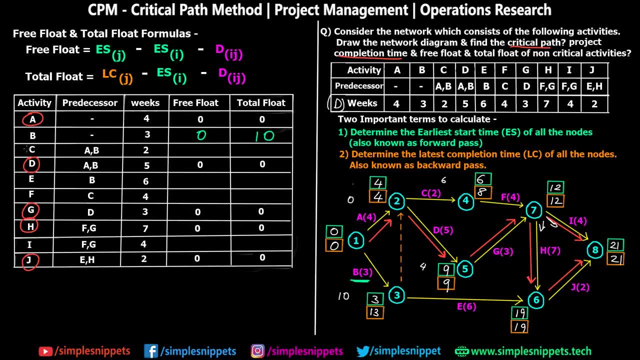 is going to be 10.. so i'm going to write 10 over here. so let's calculate this for c activity. that is this activity. so when c is involved, we have two to four. so applying the formula for free float, es of j, es of j is six. that is, this is six minus es of i, so es of i is four. 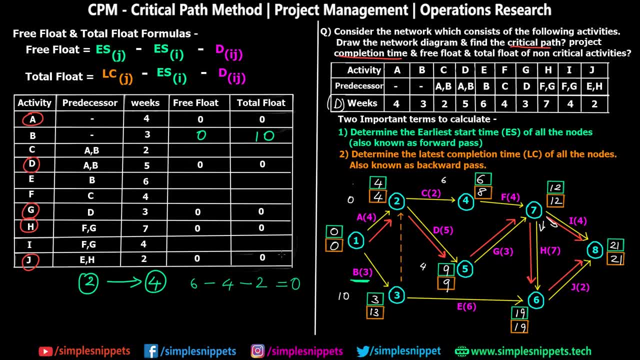 minus the distance between them, that is two, that is going to be zero. the total float is going to be lc of j, which is eight minus es of i, which is again four minus the distance again between them is two. so eight minus four minus two is going to give you. 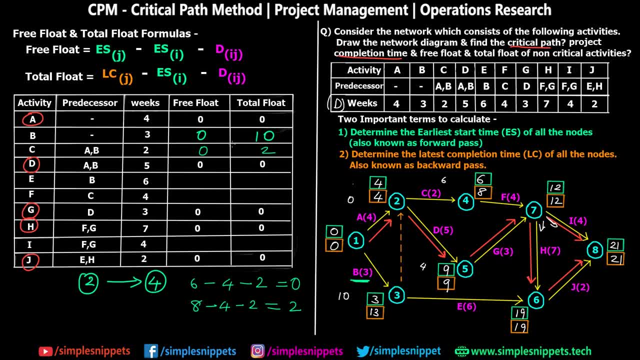 two. so this is i'm gonna write two now. similarly, you can calculate the free float and total float for all the values. i have already calculated them, so let me just directly show it to you. this is very basic formula. you just have to apply this formula and you just have to have